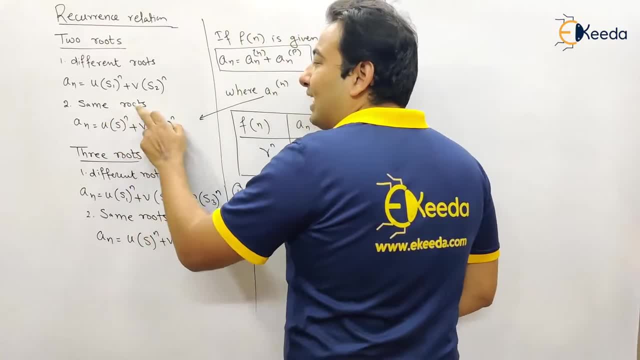 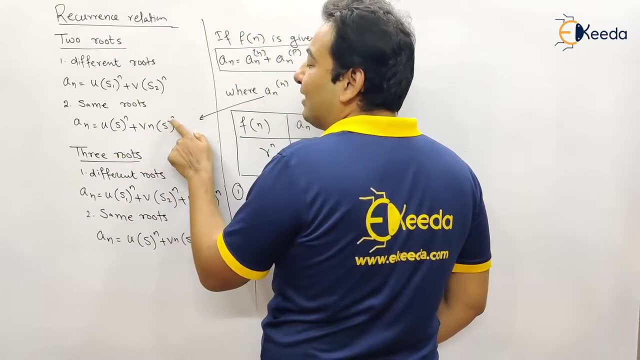 s1 and s2.. Here the roots are same. That means only one root. Since the root, only one root- we have u s raised to n plus vn s raised to n. See the format that we have Now. the root vn is zero. So s1 raised to n plus vn, n is one root. Now we have two routes. 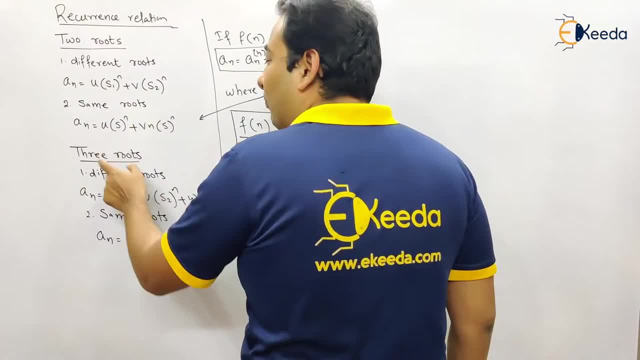 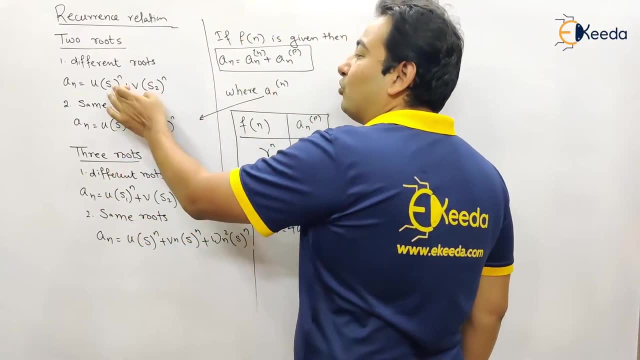 Here it is n raised to zero, Here it is n raised to one And here there are two different roots. Suppose there are three different roots. Again the same category, Three root, different root: s1, s2, s3.. So extension u s one raised to n, v s two raised to n and w s three raised. 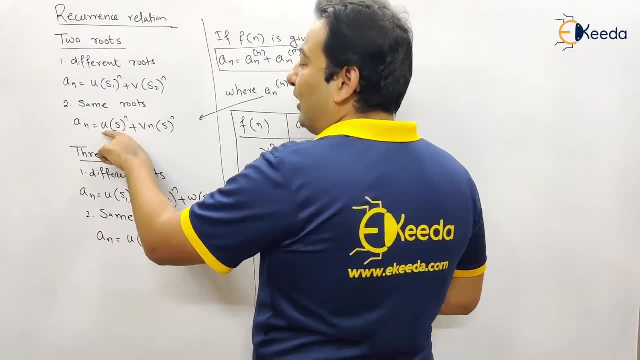 to n And suppose we have same root, only one root, That is, u s raised to n, vn s raised to n, Here n raised to zero and here n raised to one. Now n is squared, so w and N squared. 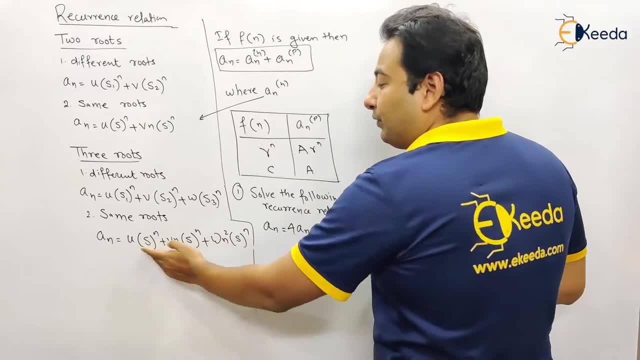 S2, n is square, soiform ay, and therefore no n is square, d2 to d2s square. So why don't we put makes a possible singular custom entry, and if the root is also a fixed cautiov, that raised to nc here. so you need to remember this particular solution. if f of n is given, then 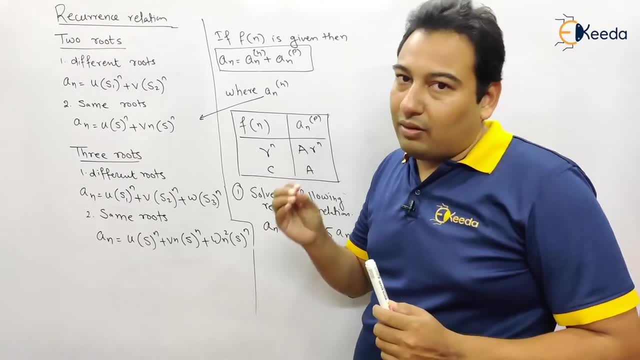 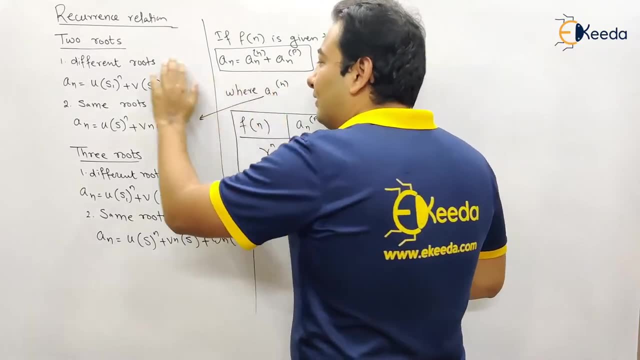 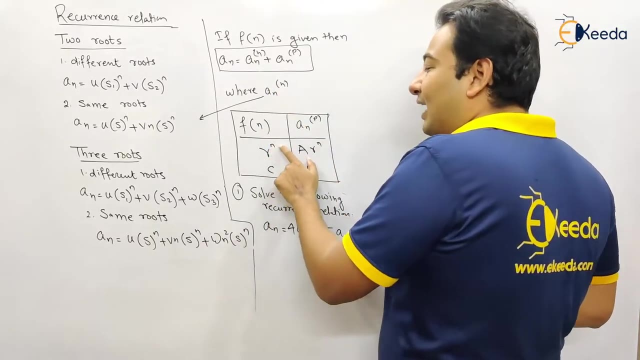 f of n is not compulsorily will be there in the problem. if it is there, then your solution is a n h plus a n p. in that case this becomes your a n h. and for finding a n p, this is the table. it depends upon the function. if the function is r raised to n, then a n p is a r raised to n and. 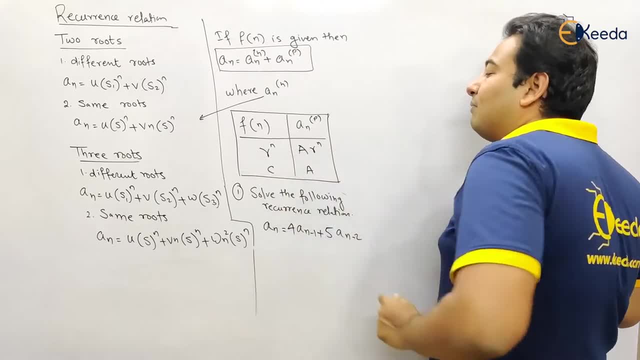 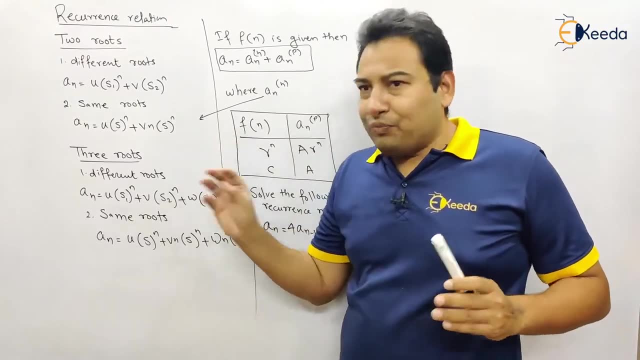 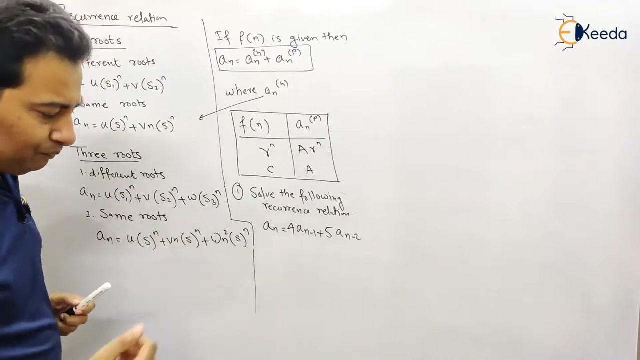 if the function is c or a constraint, you can say: then a, n, p is a. so this is the whole story. so we just discussed what is there here. just a formality. i know you didn't understand anything, so just don't worry. with the help of example it will be very clear. so let us start our problem. 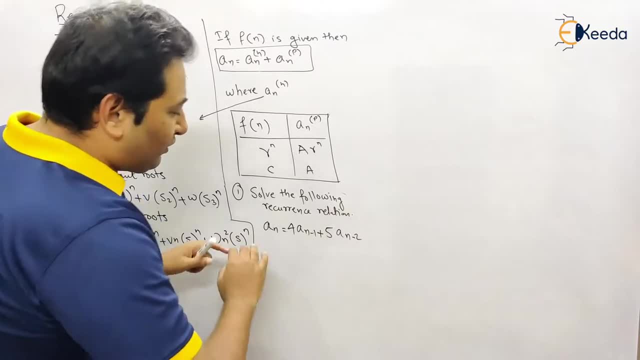 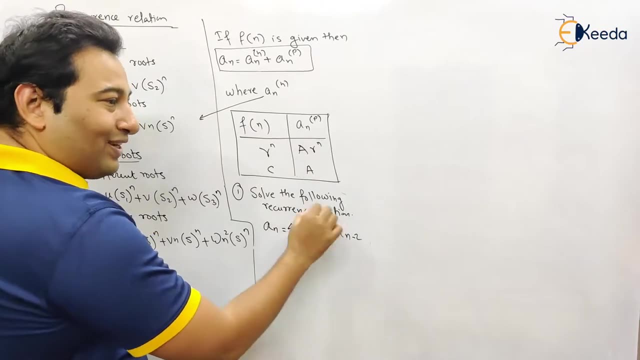 is to solve this particular recurrence relation as discussed. i've explained you why this is called recurrence relation: n? n minus 1. n minus 2. a? n is represented with the help of the same function: a? n? p is a recurrence relation n? n minus 1. n minus 2. a n? p is a recurrence relation n? n minus 2. 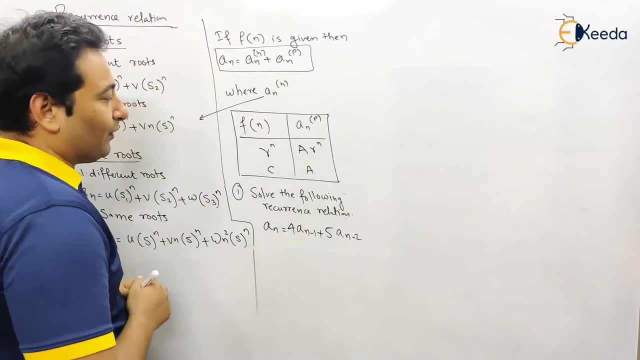 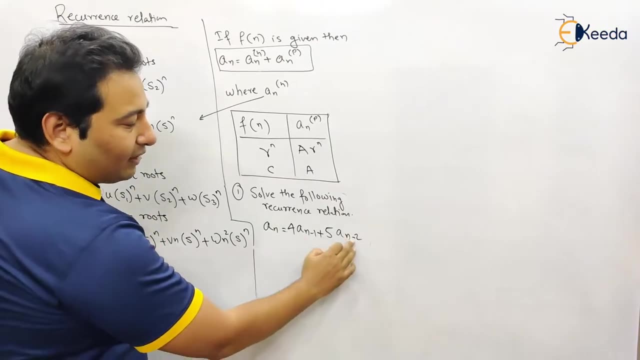 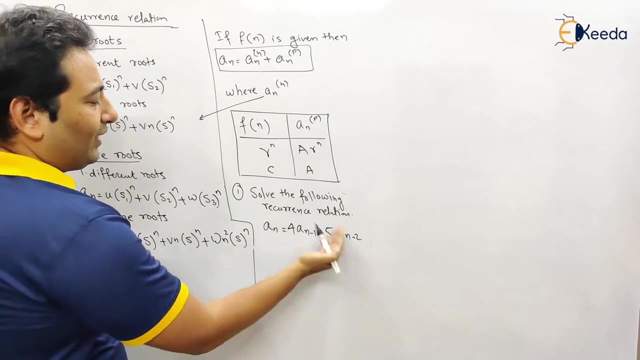 a, n, but previous two values. therefore it is called a recursive function here. there is no f of n in the problem. no f of n in the problem because only a? n terms are there. when f of n will be there, i'll tell you later on. as of now, in this problem there is no f of n. let's take all the terms to the side. 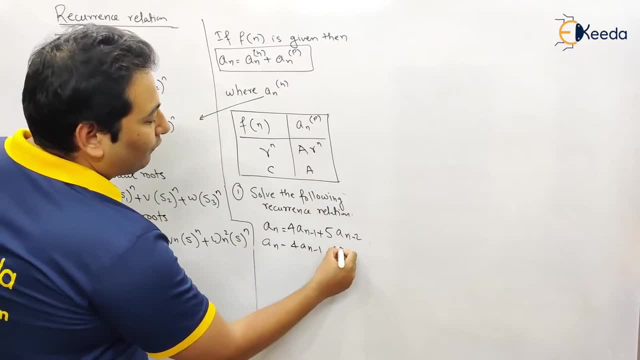 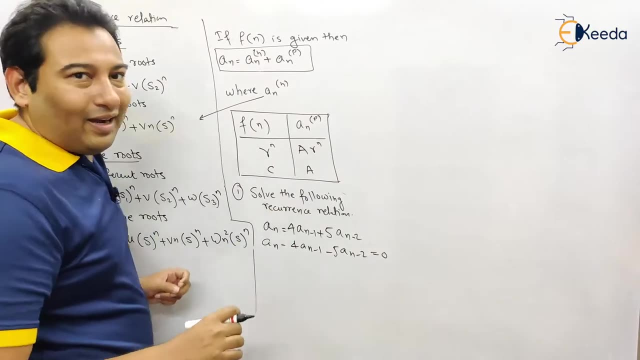 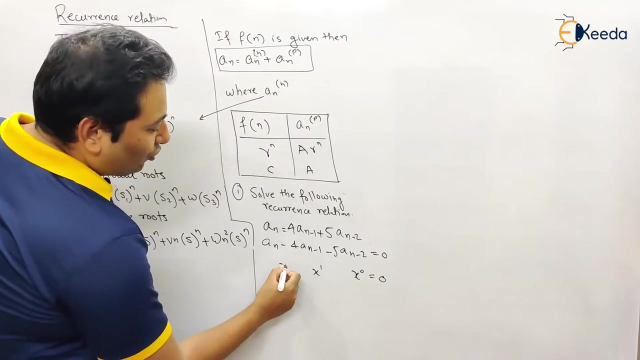 a n minus 4, a n minus 1 minus 5, a n minus 2 equal to 0. now what we're going to do? we're going to convert this equation into quadratic equation in terms of x. so here, x raised to 0. here i'm going to write it on: x raised to 1 and x square. 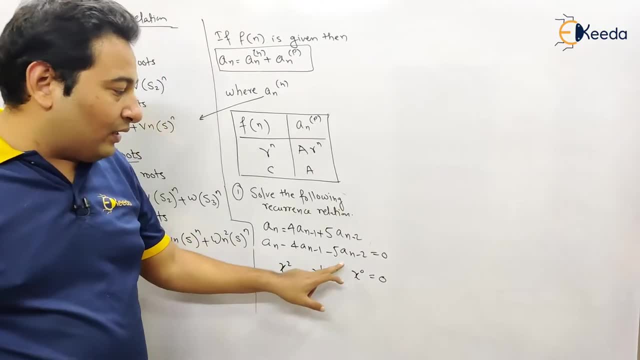 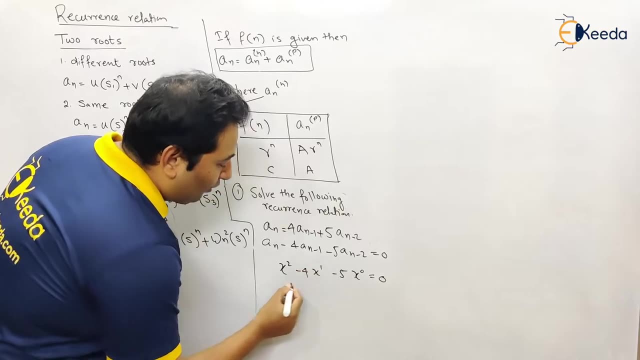 x raised to 0, x raised to 1, x square with a of n minus 2, we have minus 5, so minus 5 will come here with this term. we have minus 4 and with a n, the coefficient is 1, so in short, the equation is x. 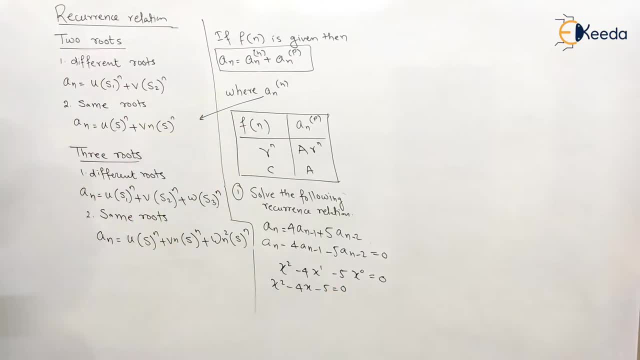 square minus 4, x minus 5 equal to 0. so this is the equation that we got. now we're going to solve this equation to get the roots. if you solve this equation, the two roots that i'm going to get is x equal to 5. 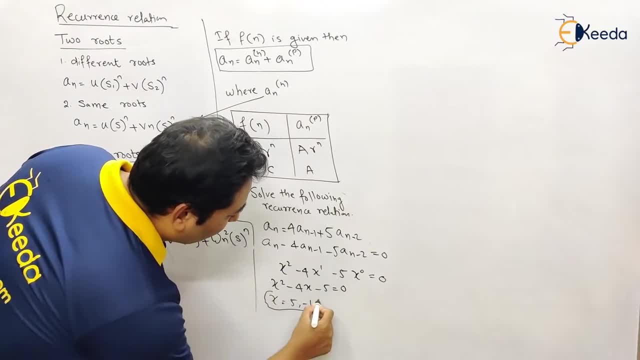 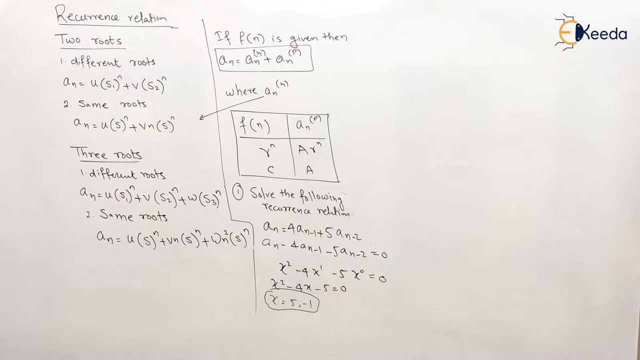 and minus 1. you put in calc and you'll get these two roots: x equal to 5 and x equal to minus 1. now we got two roots. now please tell me what is the solution? see here, for two roots. we have two possibilities with. the roots can be different or roots can be same. here there are different roots. 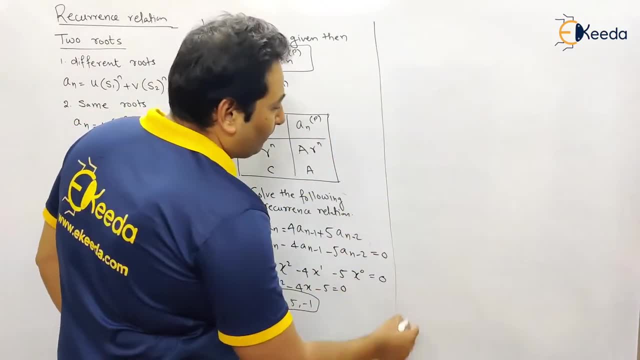 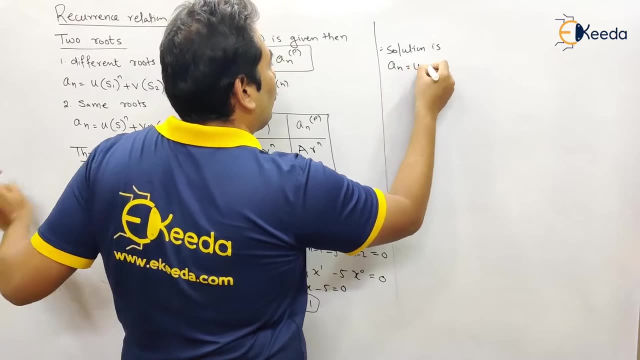 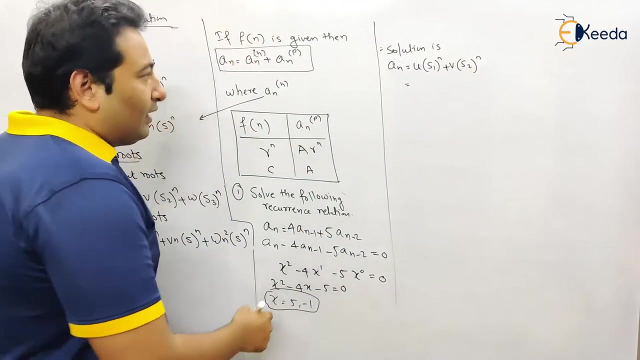 see here the roots are different. therefore, what is the solution? therefore, solution is: a. n is equal to u, s1 raised to n plus v s2 raised to n. so this is the solution. let us put s1 and s2 in this problem. s1 is the first root, that is 5, and s2 is the second root. 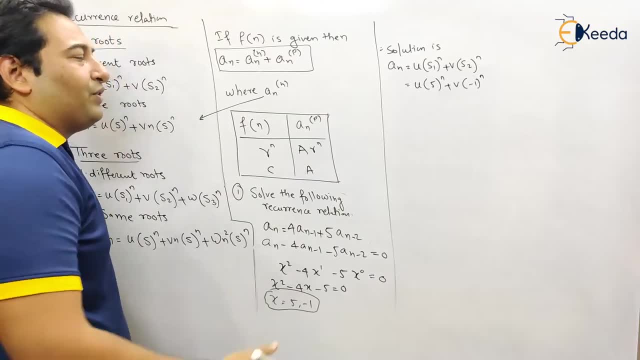 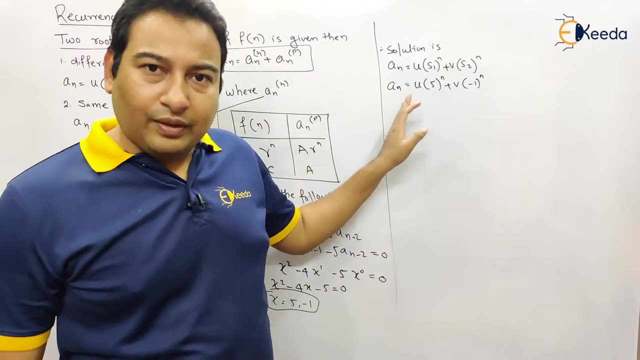 that is minus 1. obviously you can interchange s1 and s2, so no problem. so this is my required solution. it's almost done. we just need to find it out, the values of the root. so we're going to use of u and v. if we get it, the work is done. see if this is the problem given, if only this much. 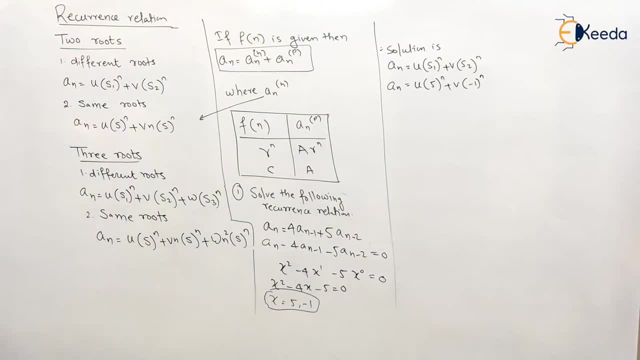 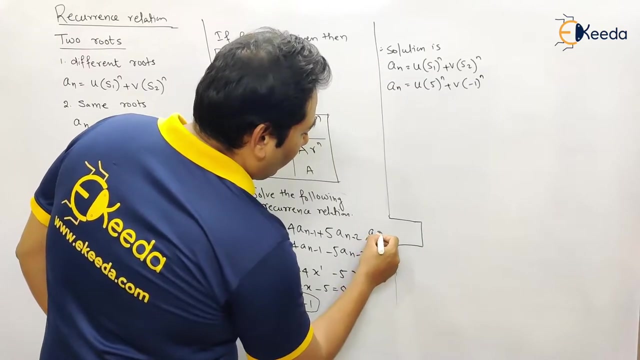 problem is given. we got the solution. that's it done. but let me extend this question with few modification. and here what we're doing is: let us let us make this problem: a1 is equal to 2 and a2 is equal to 6, so this is my problem now. 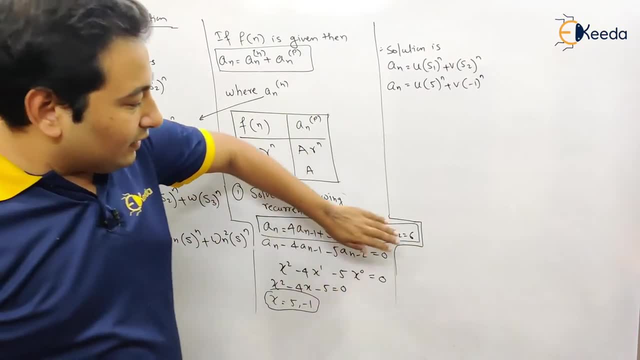 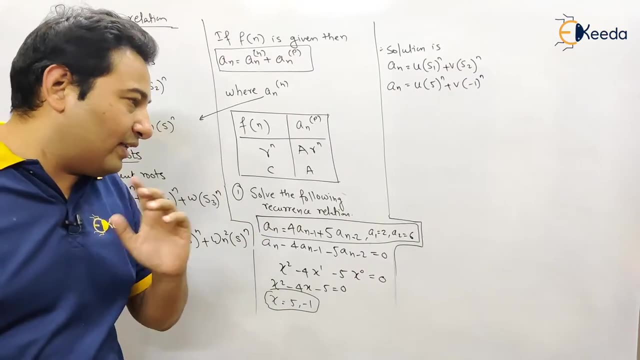 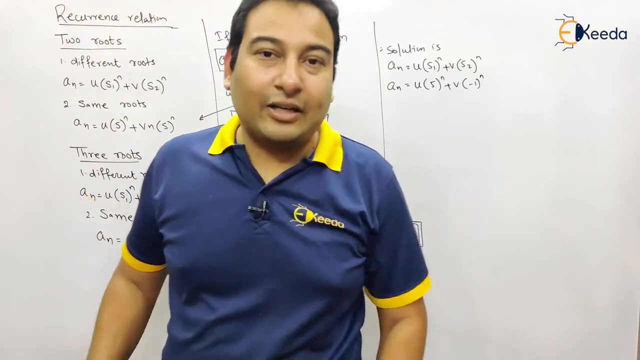 i modified my question. see, if initial conditions are not given, we are done with the problem. are you clear with this? are you clear with this? if initial conditions are not given, we are done with the problem. there were two roots. we got the solution, but if initial conditions are given, it. 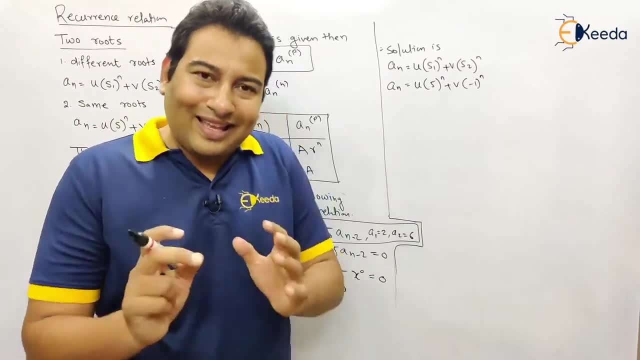 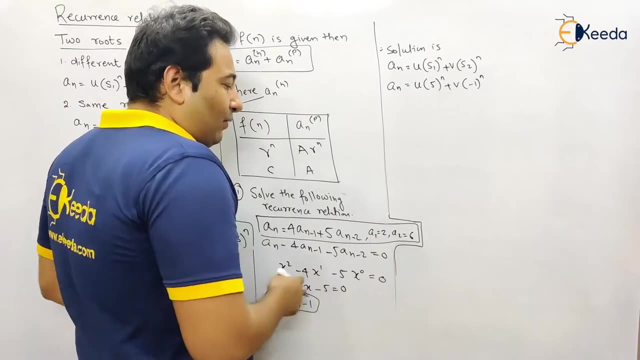 is not necessary, always will be given. it may be given, it may not be given. therefore, initially i didn't take and and we solved the problem and after that we took it. so if it is given, we need to find it out: u and v. and how to find u and v? now it's very simple, see. 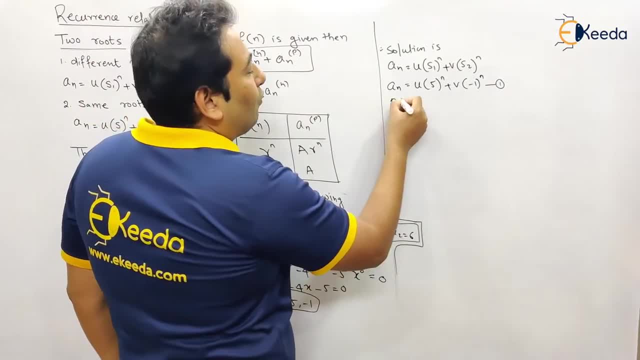 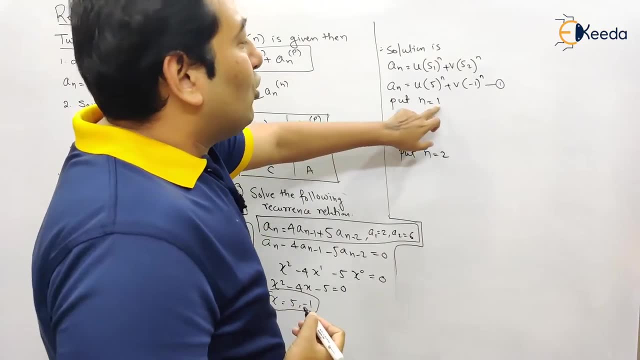 here what is given a1. therefore, we're going to put n is equal to 1 and we're going to put n is equal to 2y. if you put n is equal to 1 in this particular equation, this will become a1 is equal. 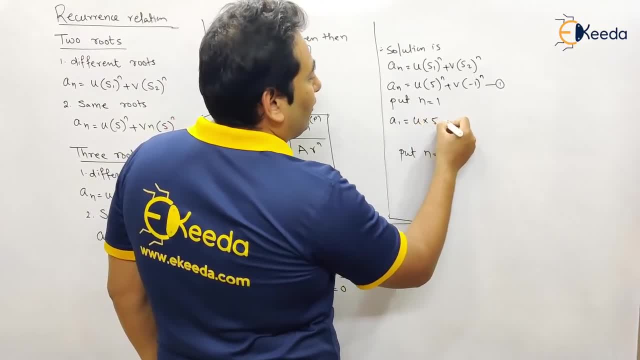 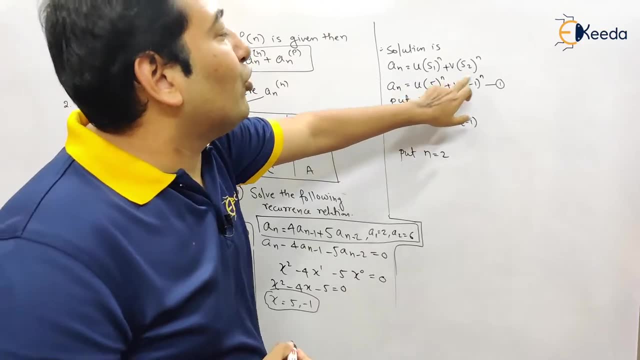 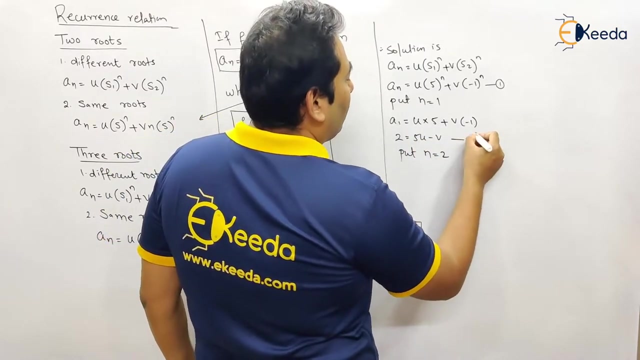 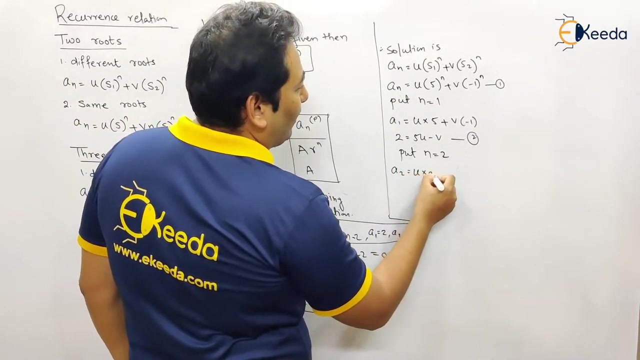 to u phi v minus 1. if you put n is equal to 1 in place of n, i'm going to put 1. and what is a1? a1 is or 2, so this is: 2 is equal to phi u minus v. so this is the first equation. and if you put n is equal to 2 here, this will become a2 u into 25. 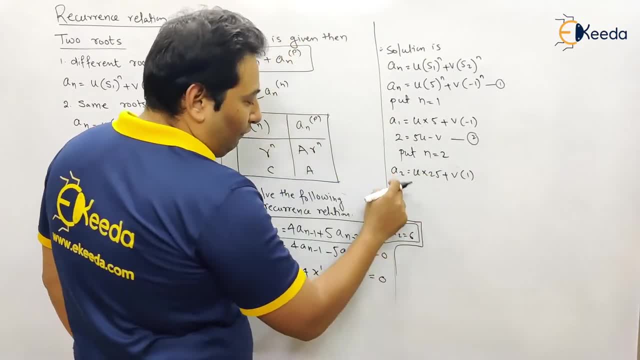 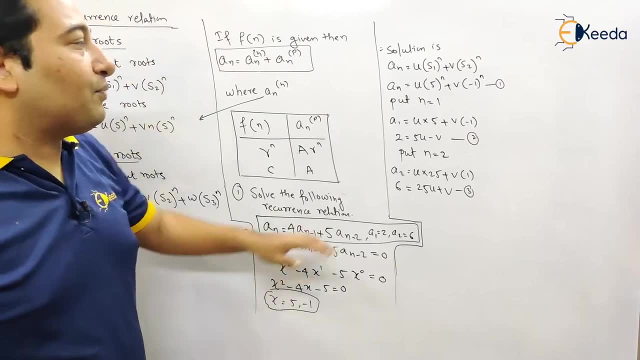 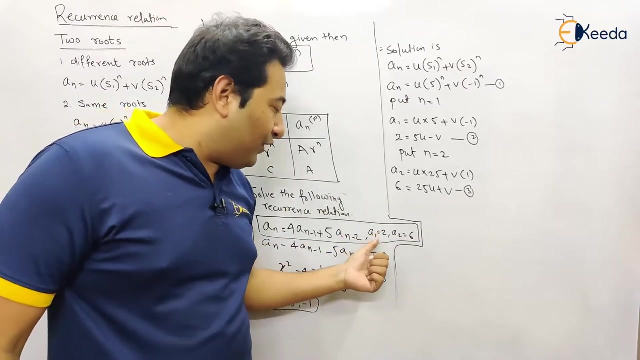 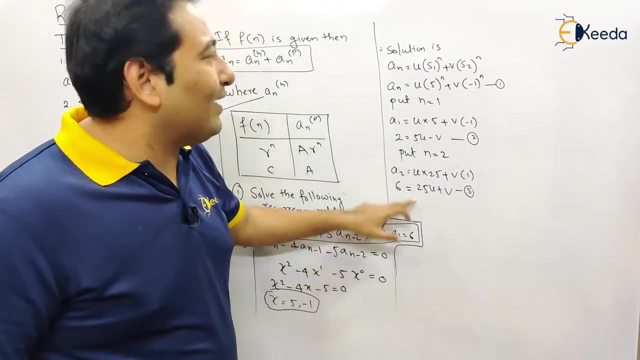 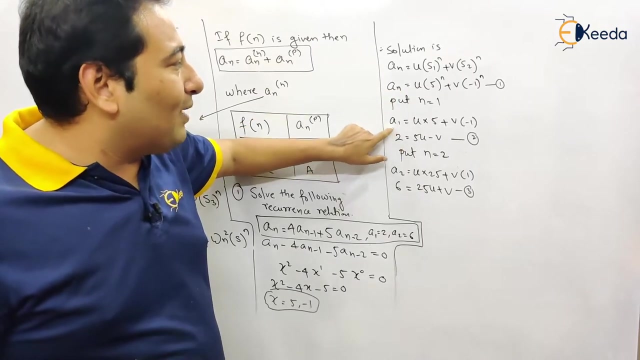 plus v into 1. so in short, if you put a2 here, this is 6, 25 u plus v. this is equation number 3. now why we substituted: n is equal to 1, n is equal to 2, because n is equal to 1 and n is equal to 2, so this will become a0 and this will become a1 and a0, a1 values. 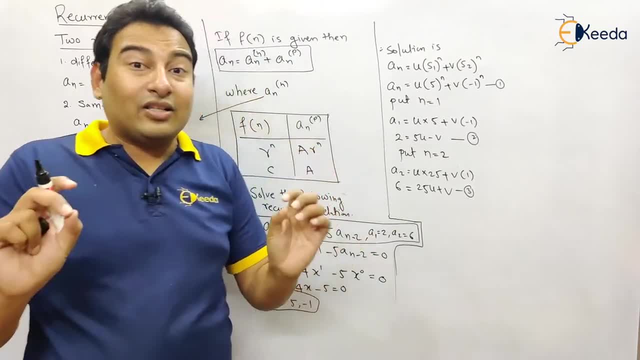 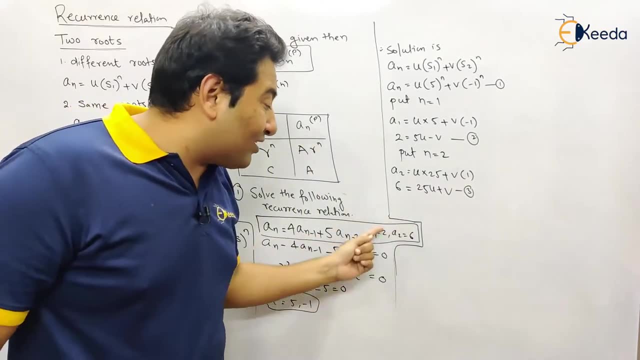 are provided in the problem. are you clear with this? why we substituted n is equal to 1 and 2 blindly. don't put n is equal to 1 and n is equal to 2. please check which conditions are given. suppose here we substitute n is equal to 1 and 2. we substitute n is equal to 1 and n is equal to 2. 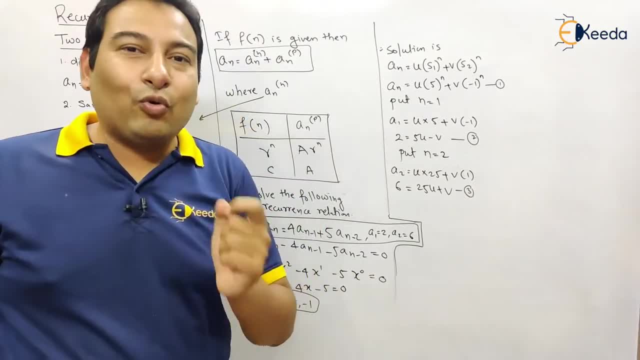 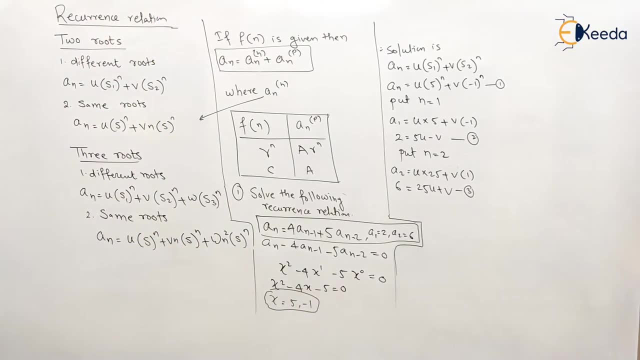 3 and 4 is given. so what you're going to do in that case you're going to put n is equal to 3 and 4. now we are ready with both the equations 2 and 3. we need to solve these two equations.